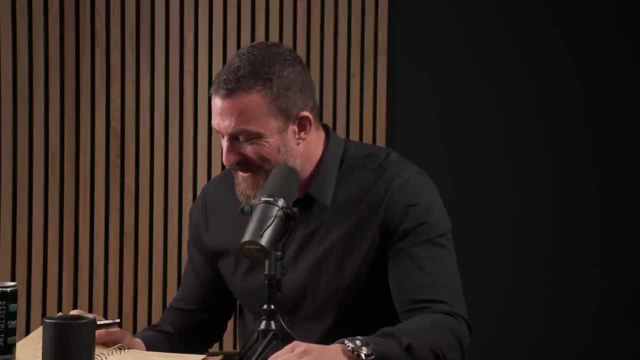 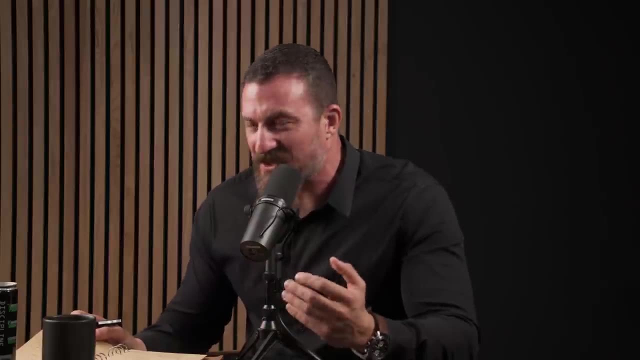 one of the most important things in the world- And I think it's a super power One that I need to focus on more. I'm- I'm grateful for bringing that up- is this is the biologist in me, but you know what is your process for engaging detachment or for disengaging. 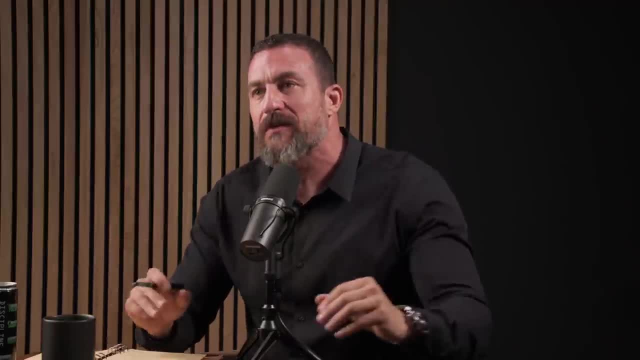 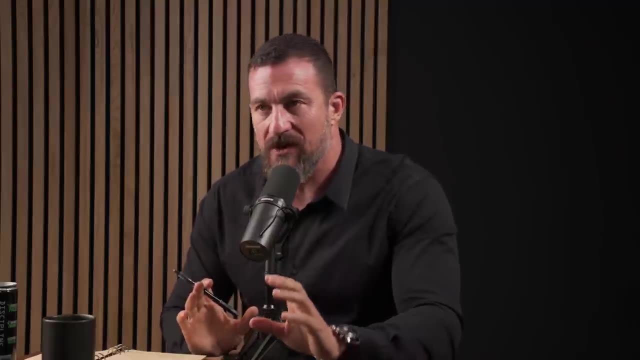 Is it an active process? where you go, you know I'm going to detach from this. I'm going to put myself in a situation that is pulling on me. There's this gravitational force and I'm going to create some imagery in my mind of walking away from it. Do I physically walk away from it? 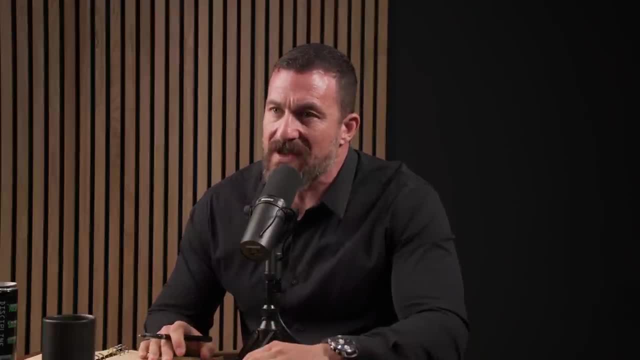 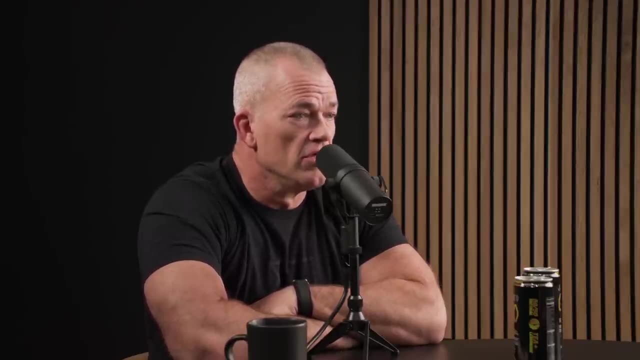 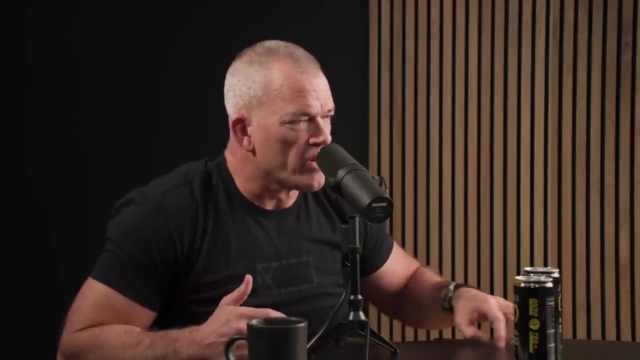 Do I outsource it to somebody else? What? what are some tools for detachment? Yeah, this is one of those situations where you and I had a discussion about the science and the practical application aligned. So my original experience with detachment was- and this is one of those moments where you know I said a lot of times- 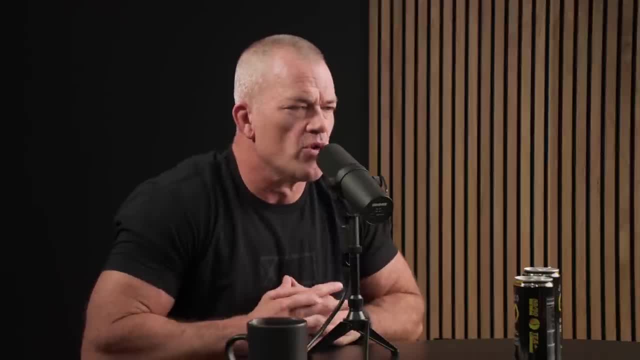 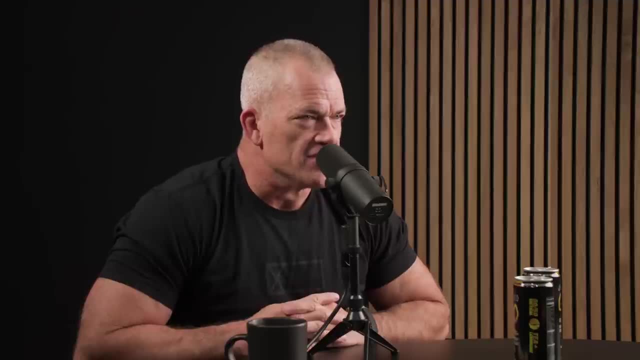 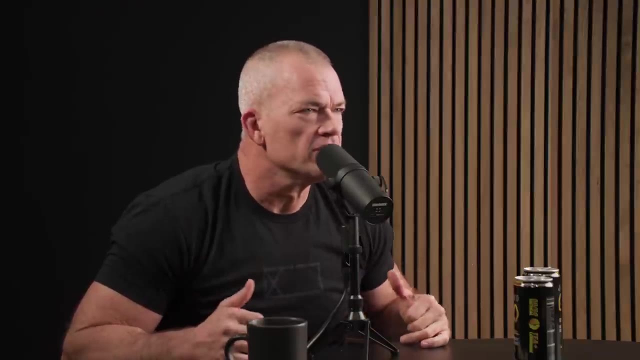 things are just small moments over time and you make a little adjustment. This is one of those moments in my life- And I wrote about leadership strategy and tactics- where I recognized, like in a moment, what detachment was and how helpful it was. I'm on an oil rig doing a training mission. 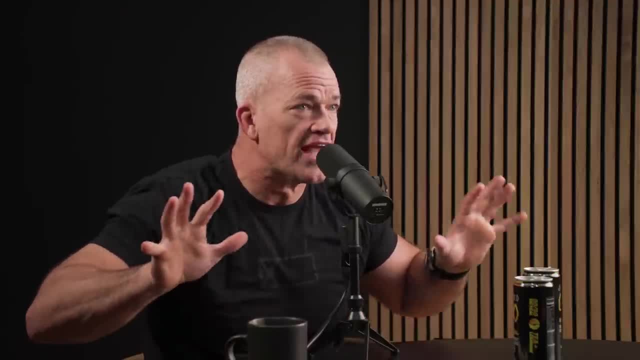 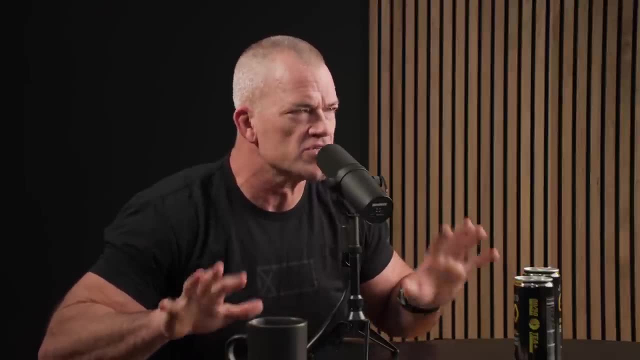 My whole platoon is in a skirmish line looking at a large area of the oil rig that we're supposed to be clearing. Again, this is not combat. This is in the nineties. There's nothing going on. We're just doing training. and I'm standing in this skirmish line- And, by the way, I'm the youngest- 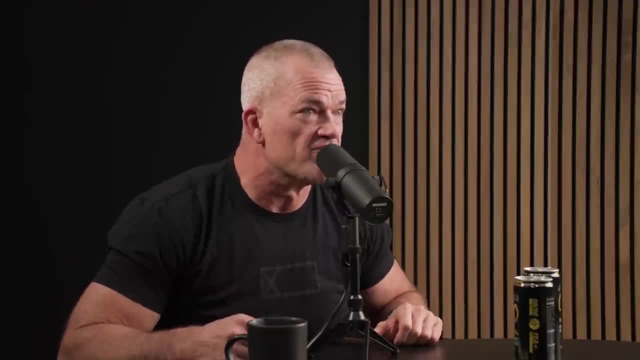 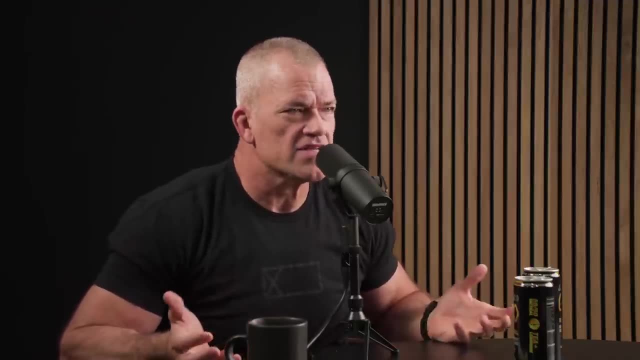 and most junior guy in my platoon And I'm standing there looking down the site of my weapon and I'm waiting for someone to make a call and tell us what to do, And I wait for five seconds and I wait for 10 seconds and I wait for 20 seconds and no one's. 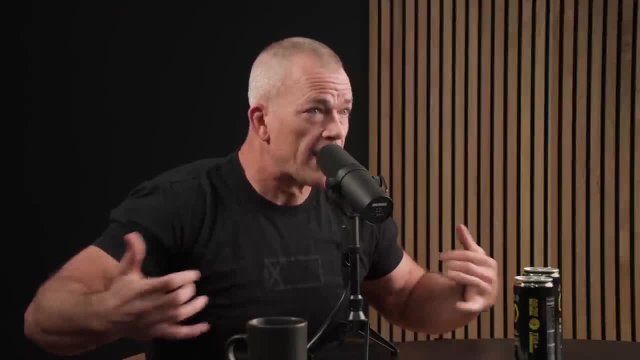 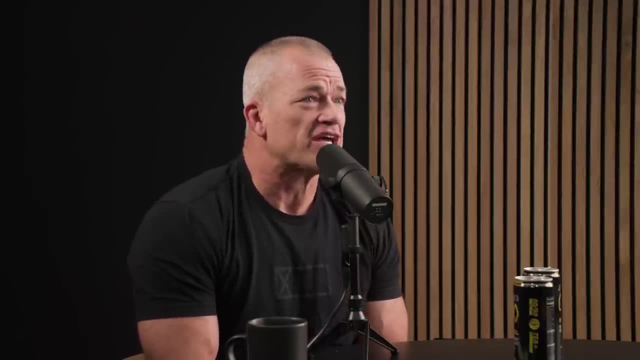 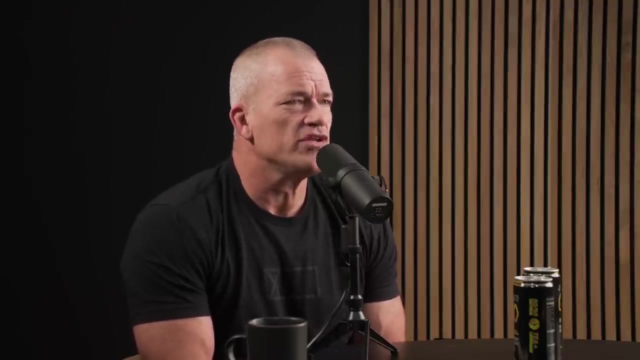 saying anything, And we're waiting for a leader in my platoon to make a call to tell us what to do. tell me what to do And finally, after like 30 seconds, which seems like an eternity, I can't take it anymore, And so I take a step like a, like a foot, a one foot step, 12 inches. 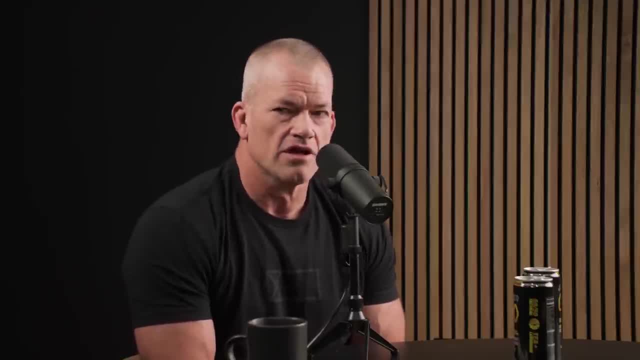 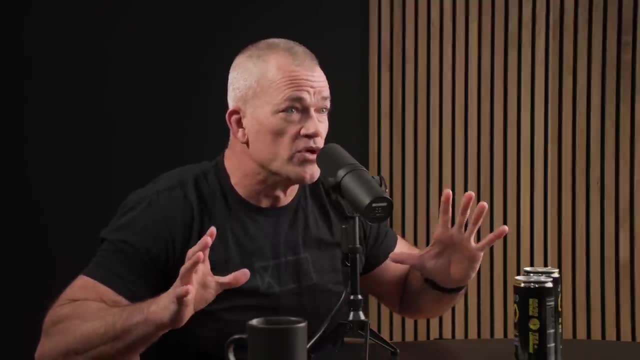 I take a step off the skirmish line, I look to my left, I look to my right And what I see is every other guy in my platoon is staring down their weapon, staring down the site of their weapon, which means their field of view is tiny. It's like a 20 degree field of view. You're looking? 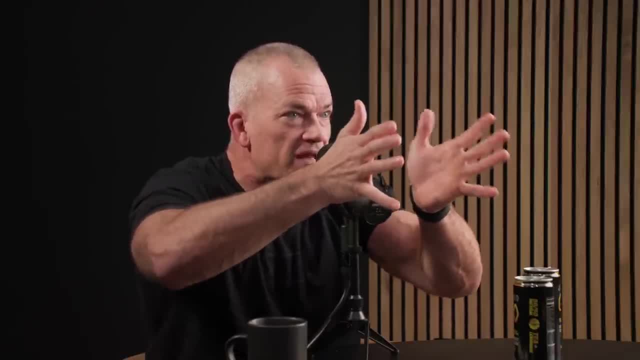 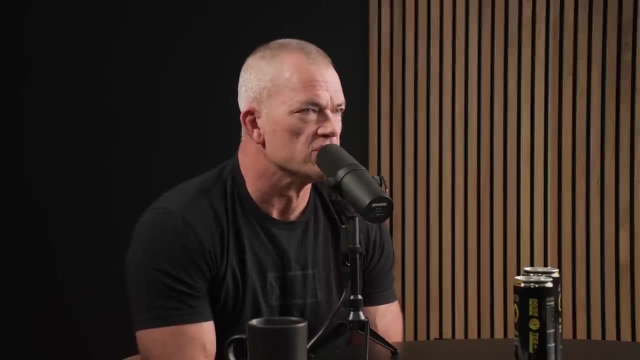 down the scope of your weapon or the site of your weapon, And that's how big their field of view is. I'm looking, I'm thinking, oh, there's my platoon commander. He's looking down the scope, the site of his weapon. There's my platoon chief. He's looking down the side of his weapon. There's my 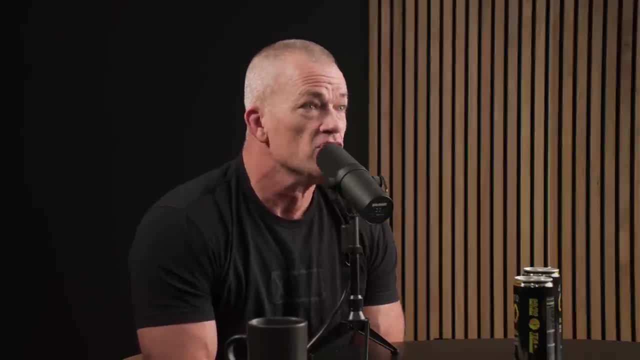 leading petty officer. He's looking down the side of his weapon. There's my assistant platoon commander. He's looking down. So everyone in the platoon is looking down the side of their weapon have a very narrow field of vision. Well, when I take a step back and look to my left and look to 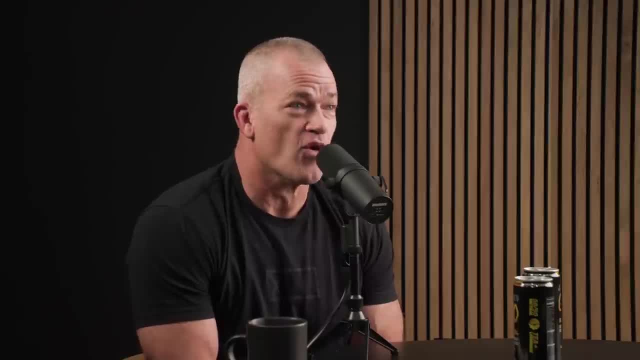 my right guess what kind of field of vision I got. I got a massive one. I can see the whole scene and I can see exactly what it is we need to do And at that moment, look as a new guy you need. 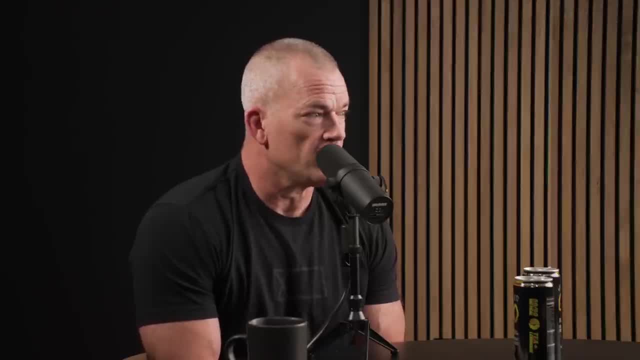 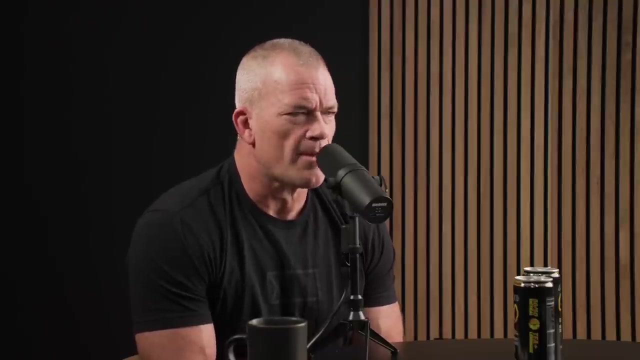 to keep your mouth shut. You don't say anything And I'm thinking well, but no one else is saying anything. So I muster up all the courage I can and I open my mouth and I say: hold left, clear right, which is a basic tactical call. No, no, no. This is not a patent level genius maneuver, It's. 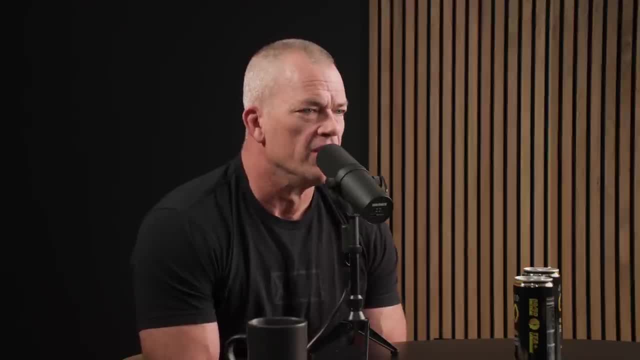 just a normal call to make in a situation that we were in. I say: hold left, clear right. And I'm expecting to get kind of slapped, told shut up new guy. But instead everyone just repeats the call: Hold left, clear right, hold left, clear right. And we execute the maneuver and we finish. 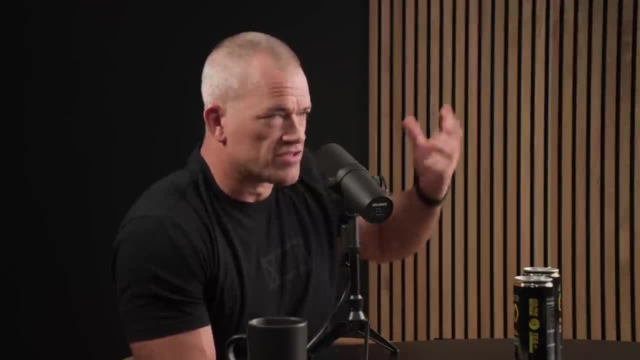 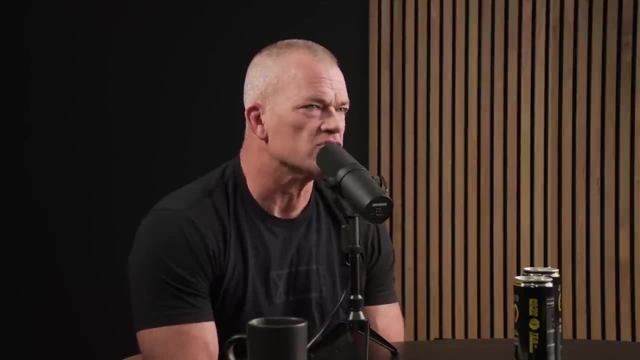 the clearance of this oil rig. And we get done. We get to the top of the oil rig, which means we cleared the whole thing. We're on the helo deck at the top and we go into a debrief And now I'm expecting. okay, now I'm going to get. 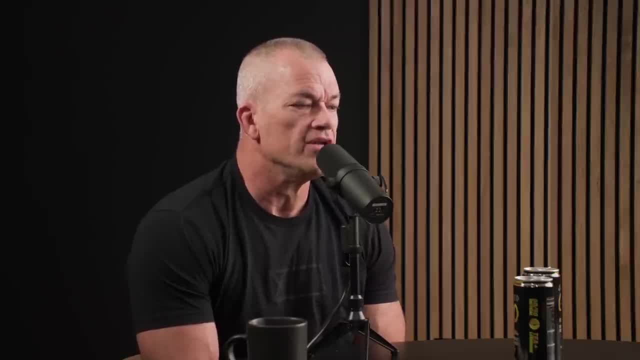 told: hey, what were you doing? You need to keep your mouth shut. And instead the platoon chief goes: hey, Jonco, good call on the cellar deck down there. And I was kind of like, yeah, that's. 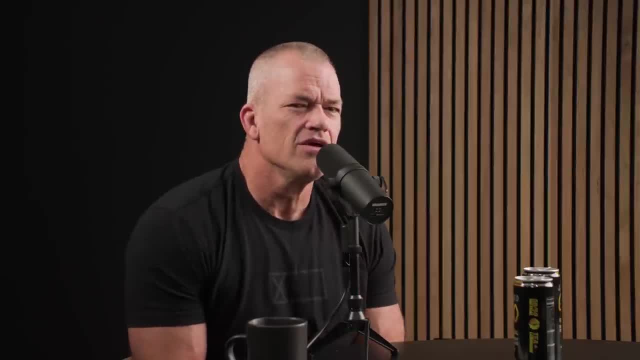 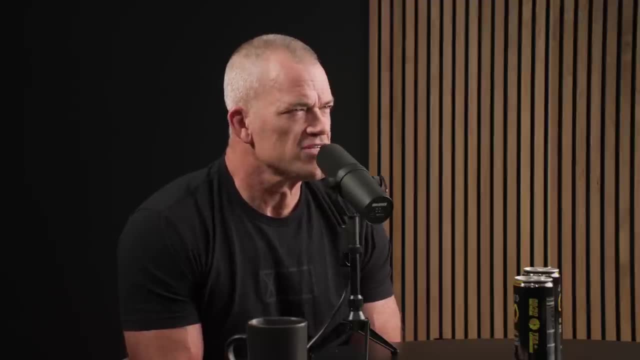 right. But then I thought to myself: hold on a second. Why, if I'm the youngest, most junior guy in this platoon, why was I able to see what we needed to do and make that decision? Why did that call? Why did that just happen? And then I realized it was because I took a step back. 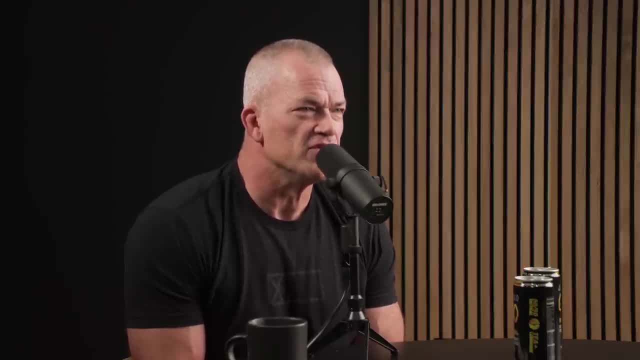 to use your term. I broadened my field of view, which allowed me to think more clearly because, instead of being hyper-focused and narrowly focused, I broadened my range of vision. I took a breath before I made my call. right, I had to take a nice breath to speak clearly. 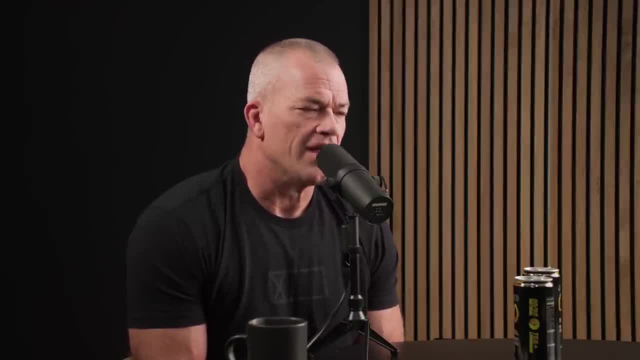 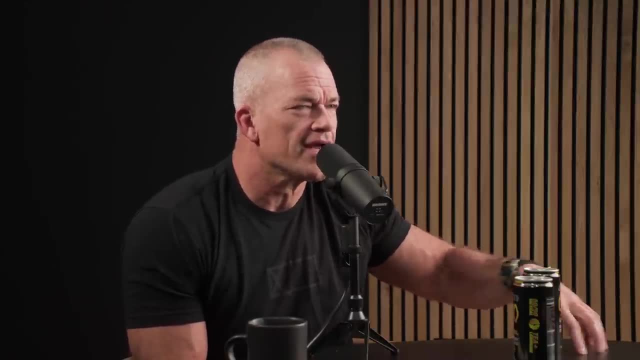 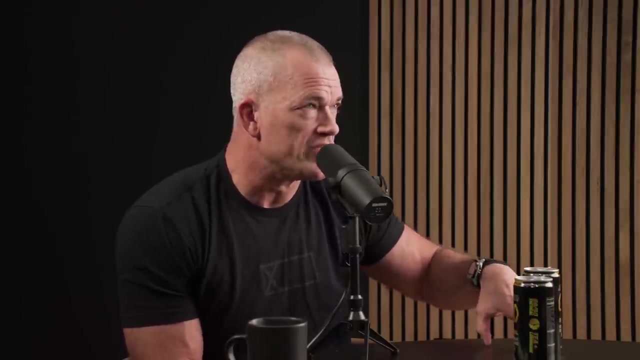 And I realized that, taking a step back and detaching, I got to see infinitely more than even the most experienced guys in my platoon And I started doing it all the time. And I started doing it in land warfare, I started doing it in urban combat, I started doing it in all these tactical training scenarios. These are 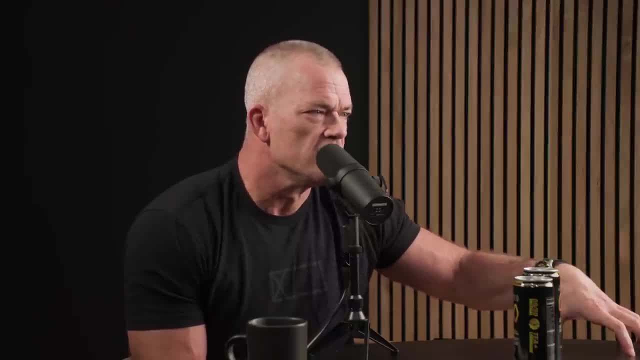 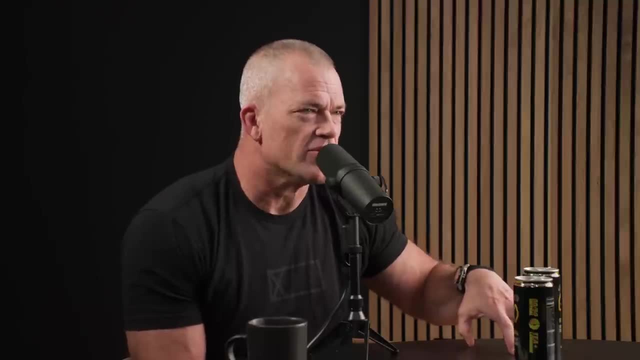 just training. This is the nineties. I started doing these training scenarios and it always allowed me to see what we needed to do. And then I started doing it like when I was having conversations with people and having a conversation with my platoon chief- And I can see that he's 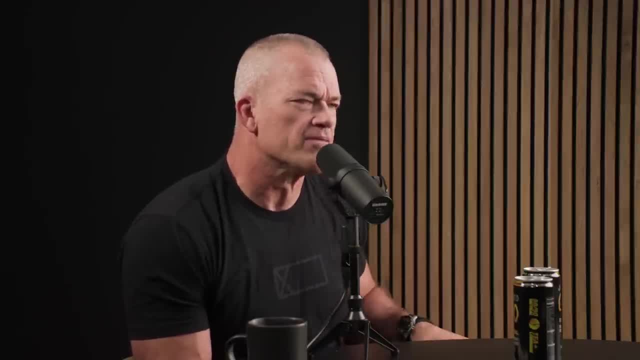 starting to turn a little red in the face, And I'm- you know we're. we're about to argue about something. I said: Oh wait a second, I'm taking a step back. Look and go, He's getting mad, right. 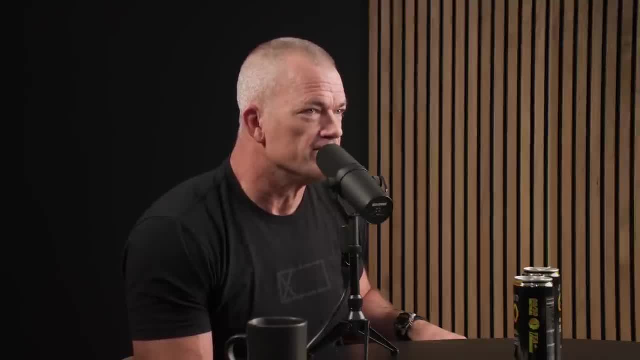 now, And he's the platoon chief, You better just deescalate this thing real quick And I'd say, Hey, you know what chief, that sounds good, Let me go take a re, let me go relook at the plan, or 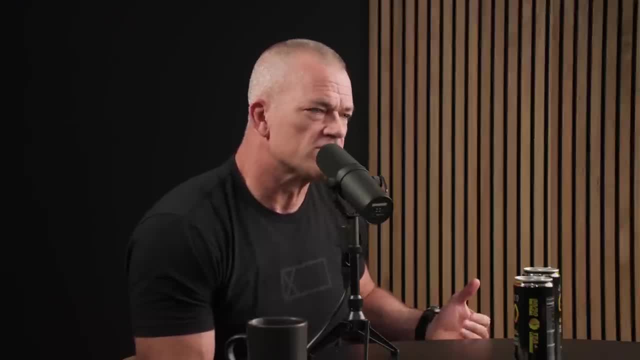 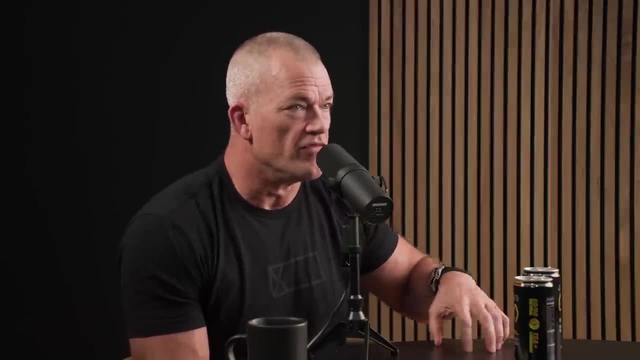 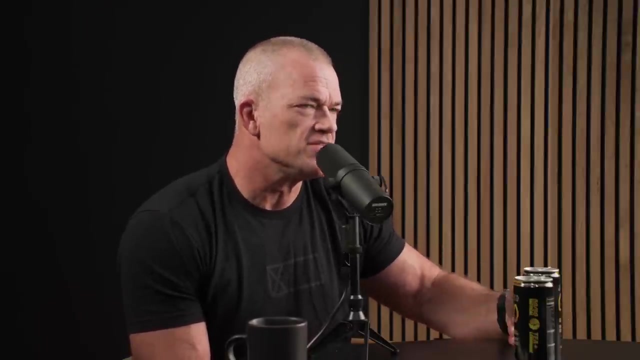 whatever. And so I started to do this kind of with my normal life was to not get wrapped up in my own emotions, not get wrapped up in the the, the gun fight that was happening right in front of my face, not to get wrapped up in the details of what was going on, but instead take a step back. 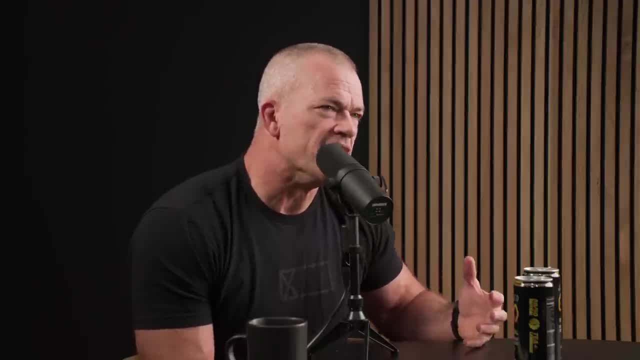 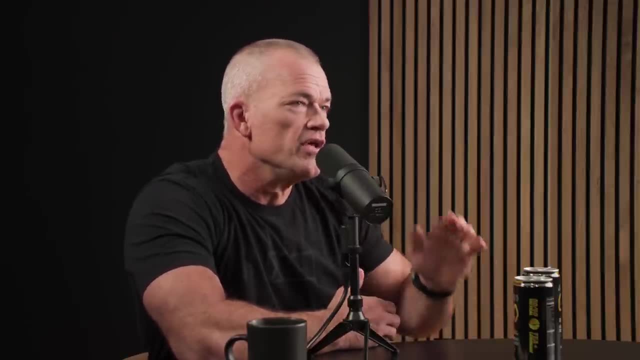 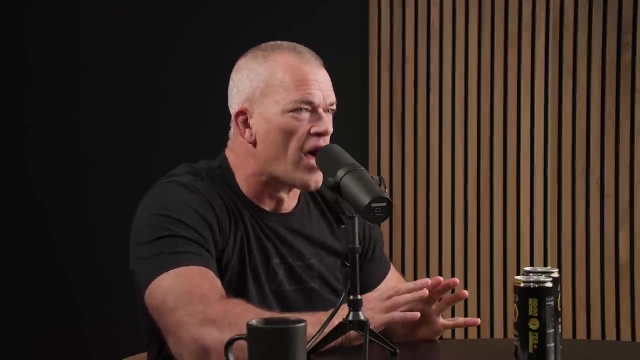 detach. look around and then you can make a bet: much, much better decision. And it's not. it's. it's exponential. You, if you're looking down the sights of your weapon and you take a step back and you look around, it's exponential how much more you can see. 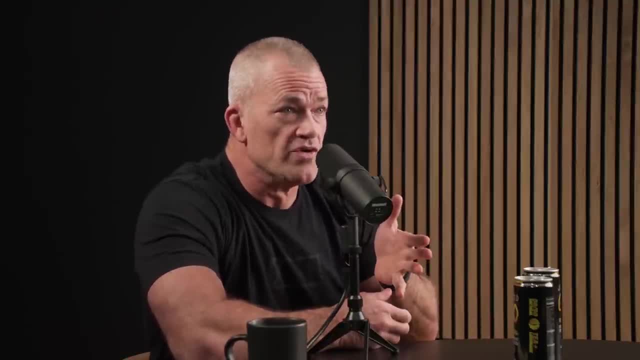 Now listen, if you are the only person in a gunfight, it's going to be harder for you to do that, because you've got to be focused on whatever you're shooting at. But when you have 16 guys or 20 guys, they're all looking in the 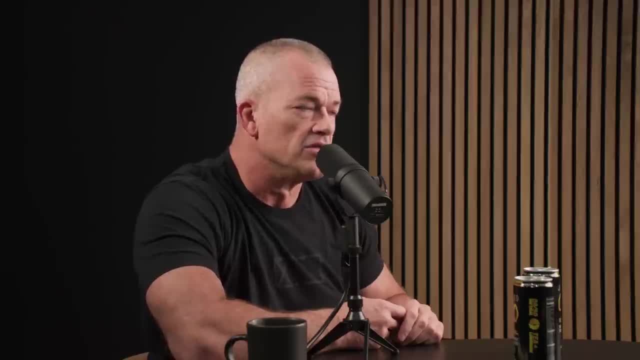 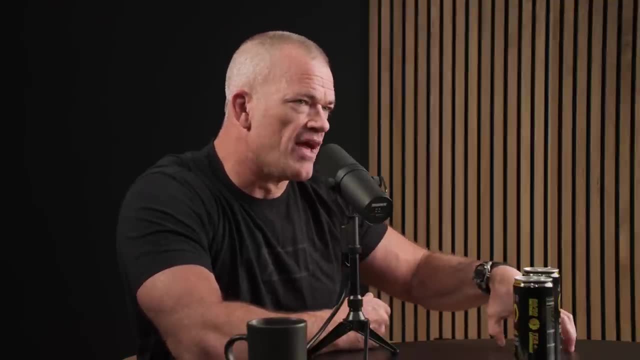 same direction. It's very easy to be the guy that goes on to take a step back. look around, make a call. So when you talk about the mechanics, when I teach this to people now, the mechanics of it take a step back. Literally. you're at. you know, you and I are at a meeting. 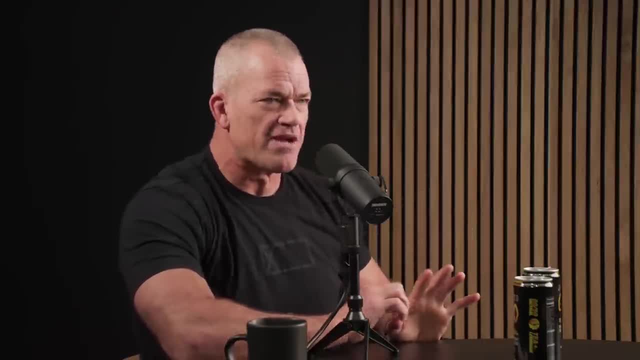 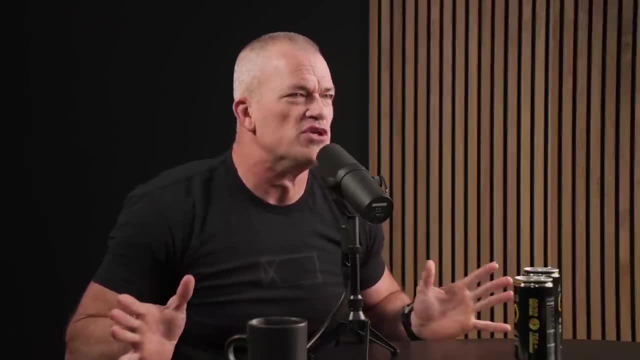 There's a bunch of people that starts to get heated argument, I will literally push my chair back away from the table. change my perspective, perspective Open, widen my field of view. The other thing, the other thing like on the in in the SEAL teams. 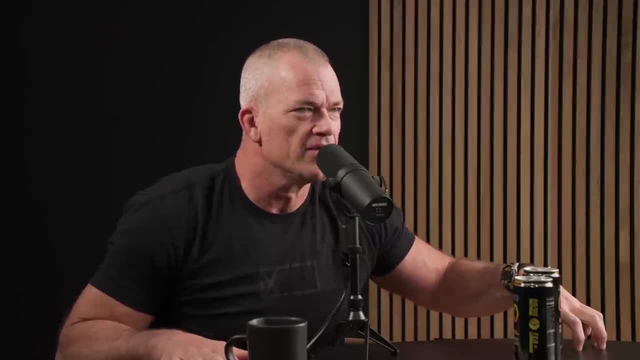 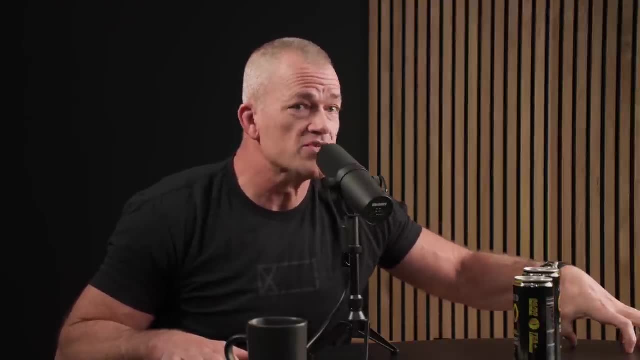 you don't want to. you don't want to sound panicked on the radio for a couple of reasons. Number one, because when you panic on the radio, it's going to cause other people to panic. Number two: if you panic on the radio and you sound panicked, everyone's going to make fun of you. 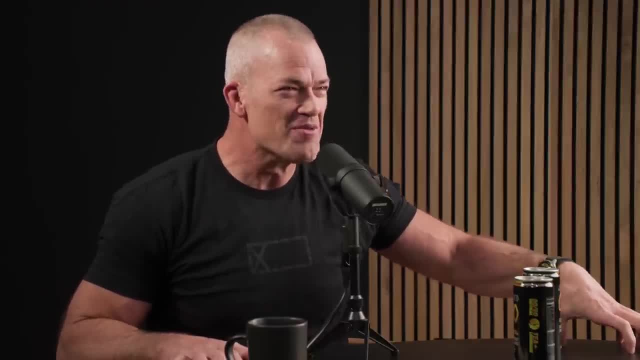 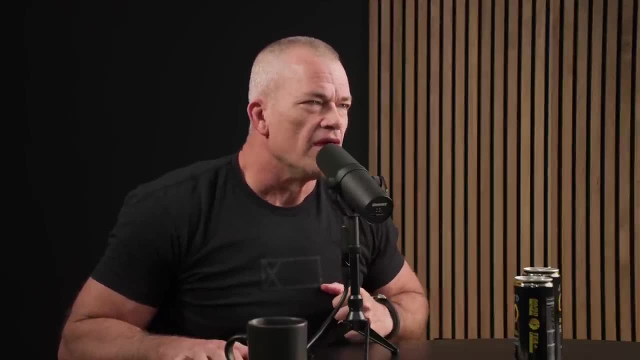 So you, you know, when you get back from the mission, everything's going to go away. Yeah, You sounded like a baby out there. So what would I do before I would key up my radio, Take a breath. So here I'm manually slowing down my breath, I'm broadening my field of view. So if you're in a 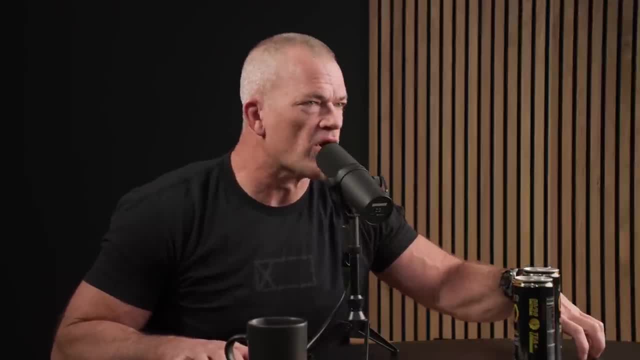 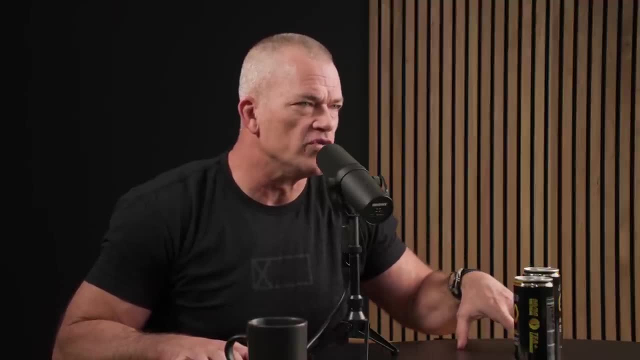 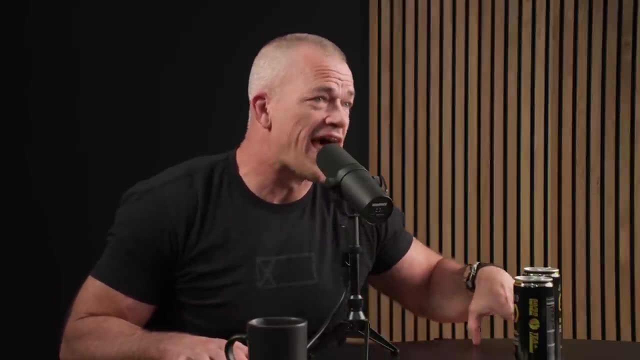 meeting or you're in a. you know you're at the, at the supermarket parking lot, and someone starts to yell at you. take a step back, take a breath, broaden your field of view, detach from those emotions that you're having and make some space. And that's that's how I go through the mechanics. 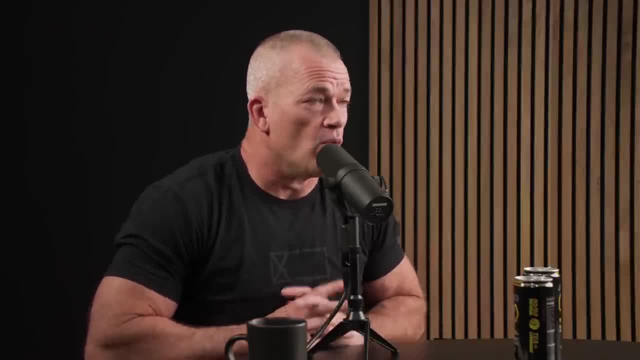 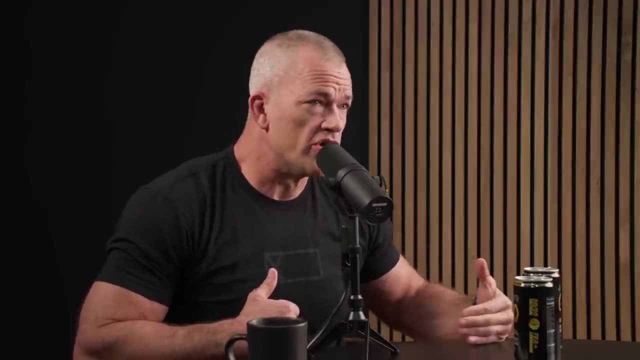 of detachment. Now I can tell you right now, I mean when, when you do this all the time- which I kind of do this all the time, I don't, I don't really have to like step back, but when you're starting to be able to try and do this. 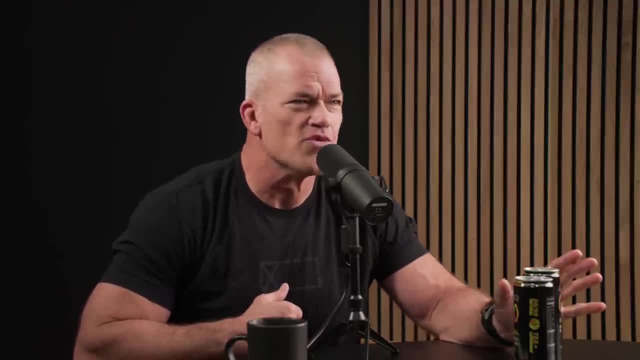 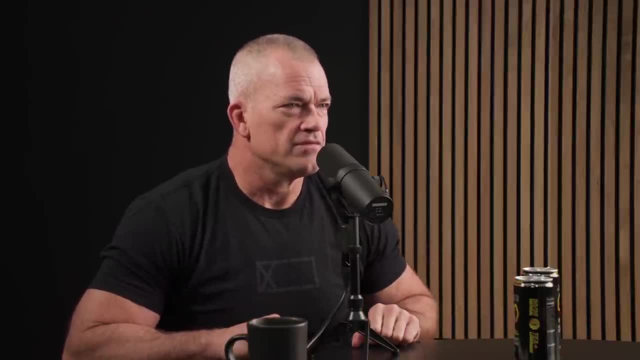 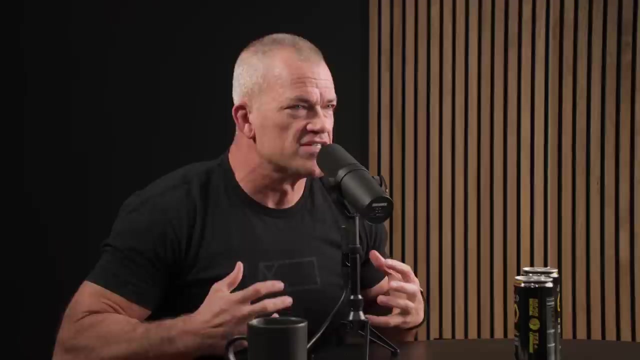 absolutely make them. And I'll tell you. here's another, like weird little nuance thing: Lift your chin up and put your hands down. Now, this isn't not in a combat situation, not in a fight, but here's the thing: When, when, when I get defensive, what am I going to do? 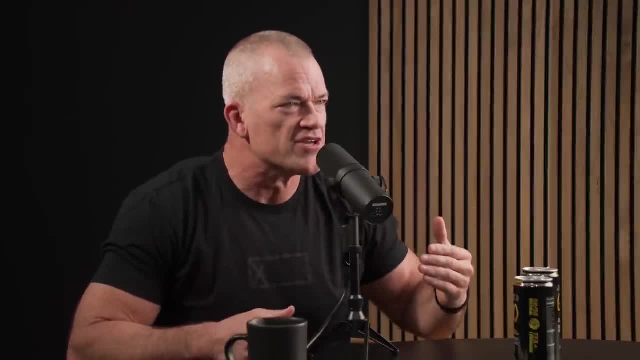 I'm gonna raise my hands up and put my chin down. That's like a fighting mode. So if you and I are having a fight, I'm going to raise my hands up and put my chin down. I'm going to raise my hands up and put my chin down. 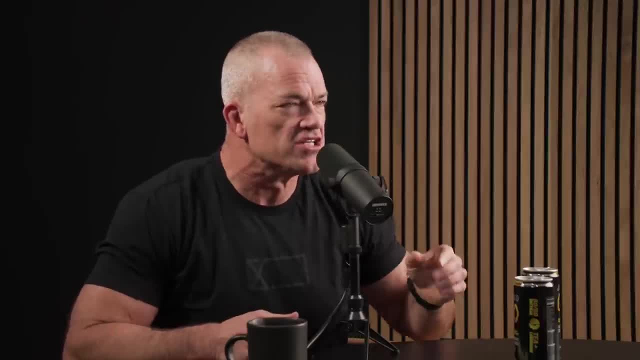 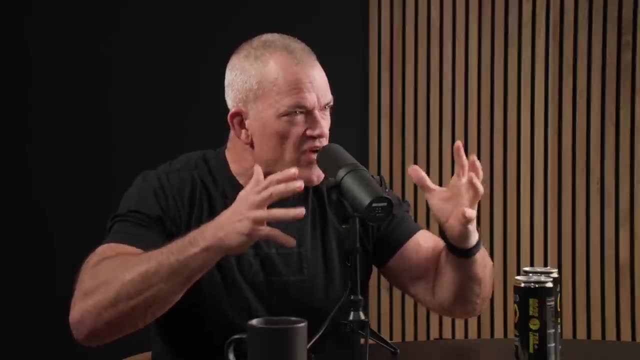 And I'm starting to get heated and I'm starting to like, Oh, he's not listening to me. instead of me putting my chin down and put my hands like up, up to where I can put them in your face a little bit, No, I'm actually gonna take a step back. I'm gonna say: put my chin up. It changes my perspective. a. 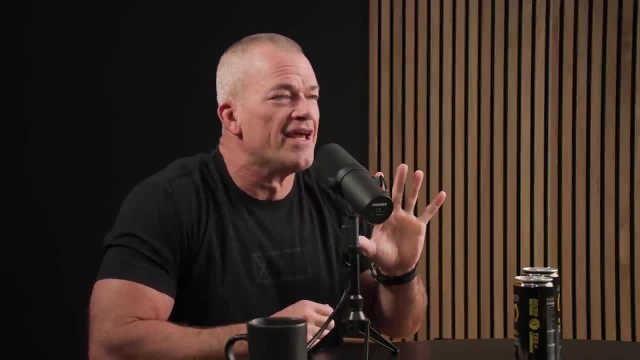 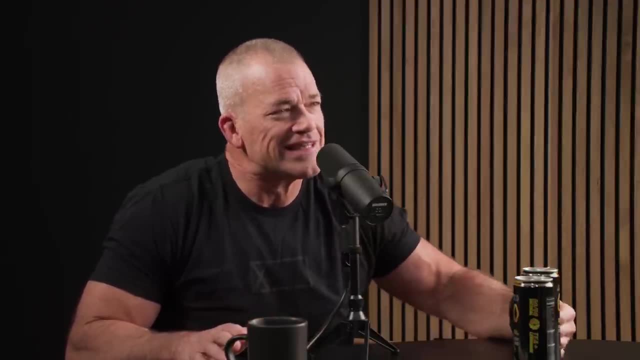 little bit more changes my visual perspective, just changing the angle of my head. Take a step back, put my hands down. I'm not being in a defensive mood. I actually want to hear what you have to say. And if I start listening to what you have to say and not talking, 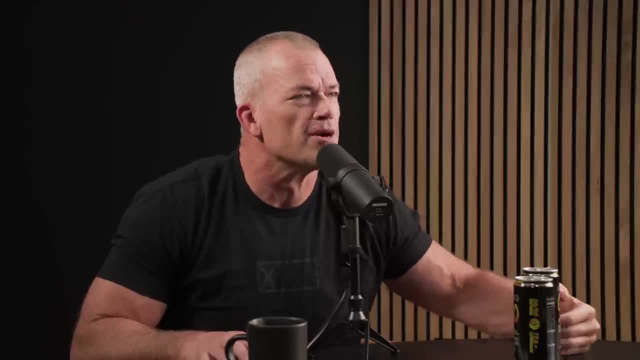 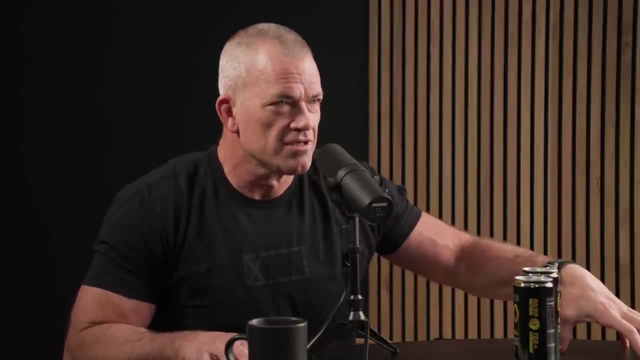 it's very hard to be detached when you're talking. It's another key component. You want to detach, shut your mouth. So I'm in meetings. you know, I'm in a bunch of different companies. I'm running a. I have a bunch of. I own a bunch of different companies. I'm in a meeting in my